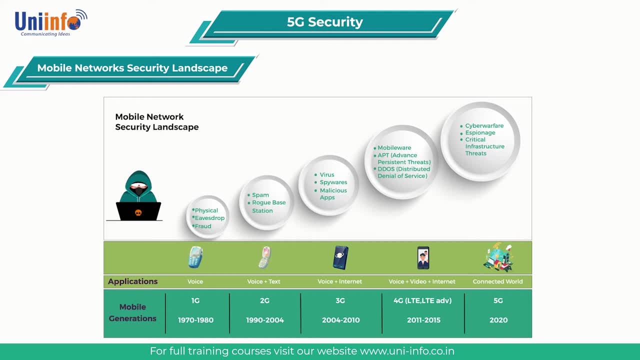 users in a single attack, or the LinkedIn 2016 breach that impacted 117 million, resulting in a leak of sensitive personal and professional data. Mobile network security has gradually evolved in parallel to the evolution of the telecommunication industry. Mobile Network Security Landscape- The mobile network security landscape as shown in the figure on the screen, should: 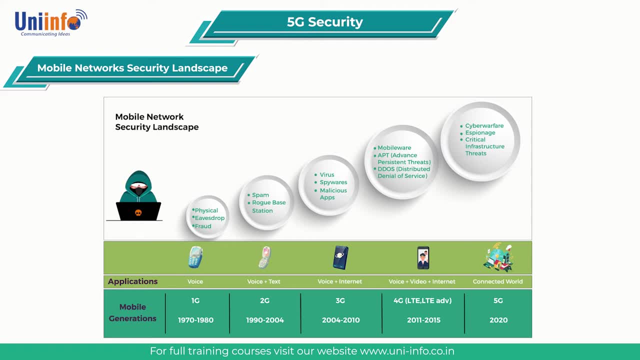 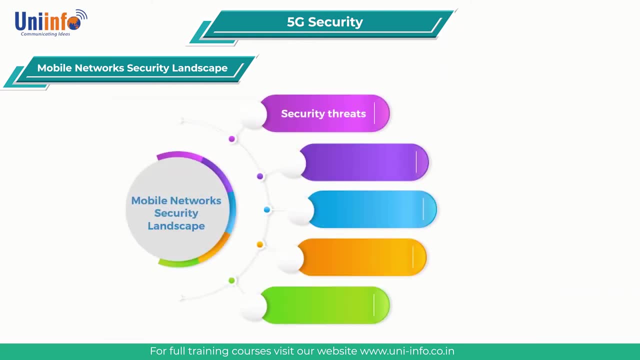 be viewed in the light of how the various generations of mobile networks have evolved. There is a direct correlation between the two In the evolution of the mobile network technology and the relative evolution of security threats in terms of the technology architecture, technical capabilities, services offered and associated. 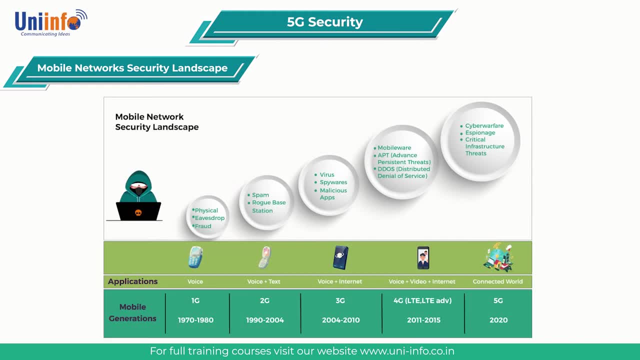 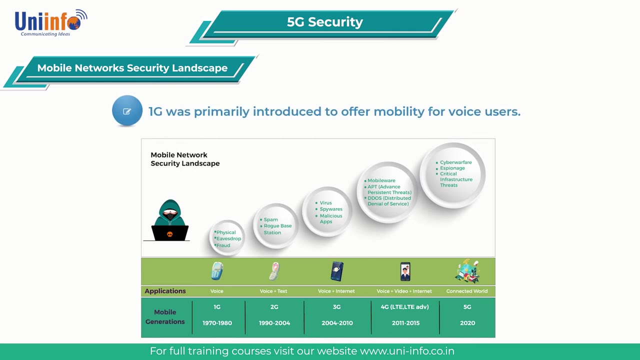 threat vectors. Mobile networks started witnessing serious threats and challenges immediately after the introduction of the first generation of mobile technology and has kept on growing as a complex and challenging threat landscape. 1G- Voices- 1G was primarily introduced to offer mobility for voice users. 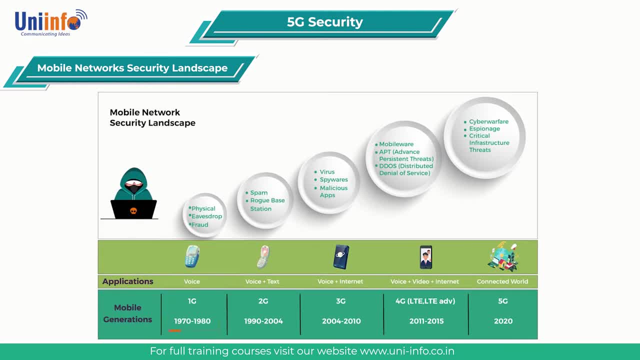 Consumers started witnessing the freedom to attend and make calls, while mobile criminals discovered an opportunity and method to commit mobile frauds and impersonate the legal subscriber to hack their phone to make free calls. Cell phone cloning became an industry by making and selling illegal cloned phones. 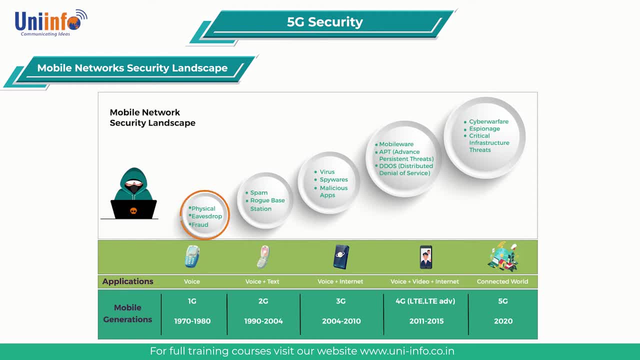 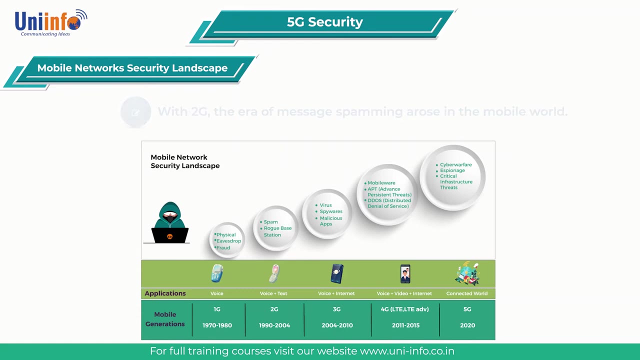 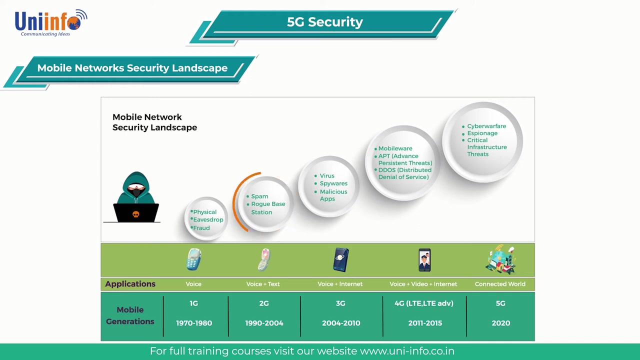 Some hackers identified new ways to hack their phones. 1G was primarily introduced to offer mobility for voice users. On the other hand, capitalism burnt out 3G. 3G gave an immediate return to the population and spawned hundreds of thousands of no-aga. 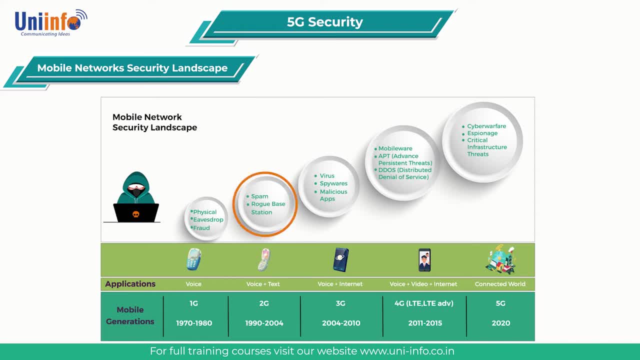 users. You could not educate yourself in 2G o1. This gave the mobile users an opportunity to catalyze the glass ceilingako 3G for the targeting a certain group or the wider community. Fraudsters used mobile spamming for their 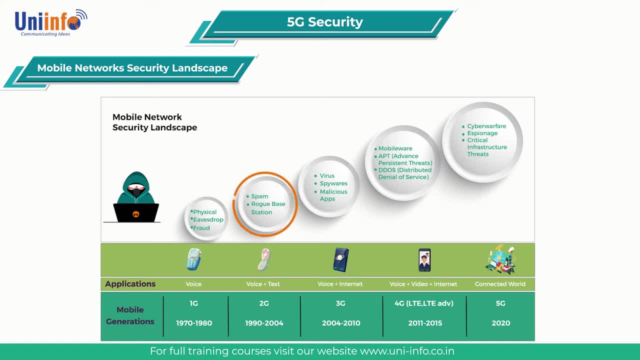 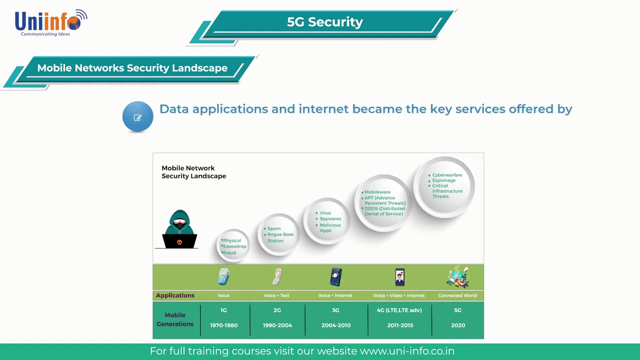 own vicious purposes. Rogue-based stations, also called IMSI catchers, were invented to intercept mobile traffic by offering fake network authentication. As the user devices became smart and resourceful, data applications and internet became the key services offered by mobile service providers. in new 3G networks, An average 3G data connection speed was somewhere. 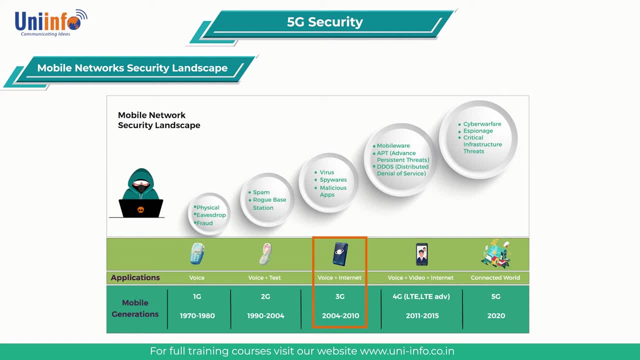 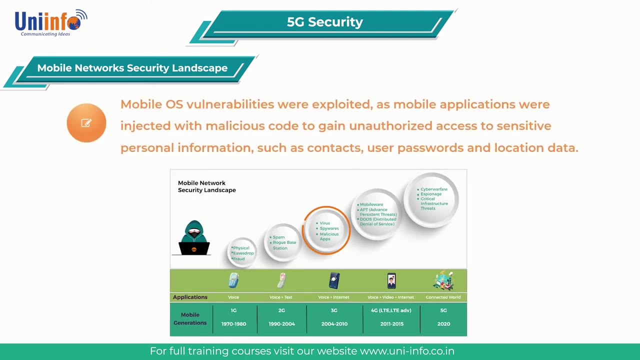 between 500 and 700 kbps, which was sufficient to provide connectivity for internet-facing applications. Threat vector in 3G targeted the user phones, computer systems and its operating system. Mobile OS vulnerabilities were exploited as mobile applications were injected with maliciously. 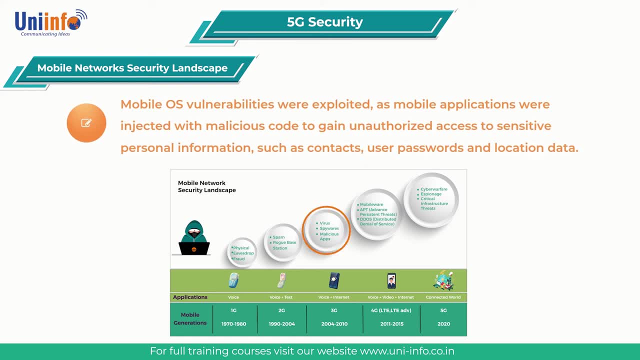 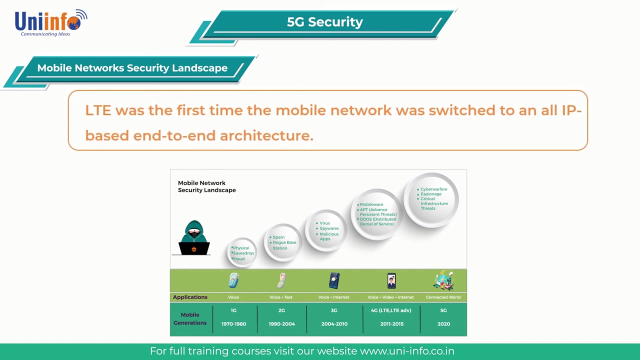 As the data speed increased, so did the type of infections in the shape of malware and spywares. LTE was the first time the mobile network was switched to an all-IP-based end-to-end architecture. It ahead to mobile service providers with speed of innovation. 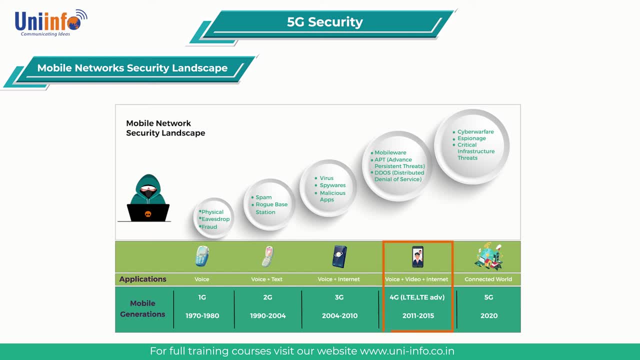 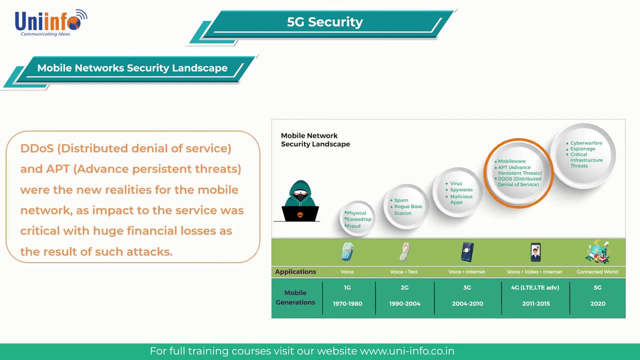 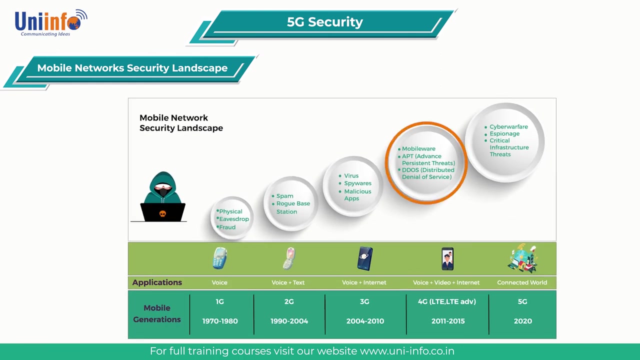 Although Intel has improved its technology, the Internet has also improved, incorporating more hardware and hardware-based hardware, such as Windows Office, Microsoft Office, Word and Apple Office, and the latest Android OS 3.. 4G, G1.. 1.- 1.. 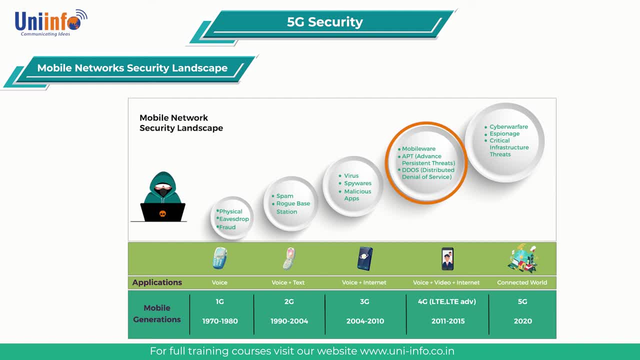 1. 2. 1. 1. 1.. It has become harder to detect their stealth presence in the mobile network, to protect and mitigate, with an average attack consisting of months' duration. 5G is coming forward with the promise of connecting billions of devices. 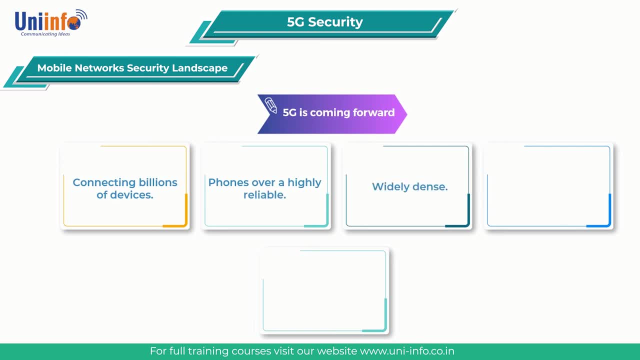 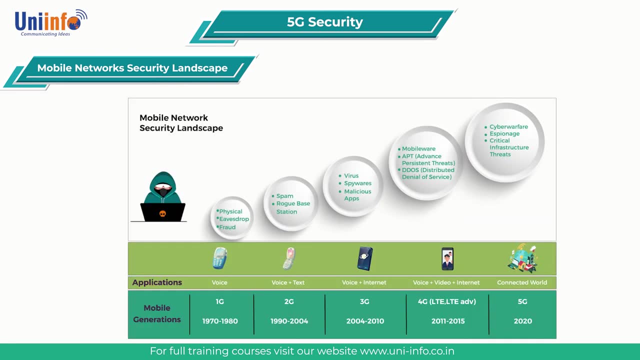 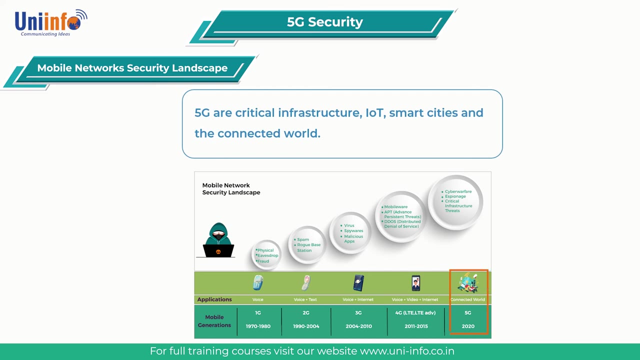 phones over a highly reliable, widely dense, bandwidth-capable, fast and fault-tolerant network infrastructure which will service multiple sectors and industries. Key use cases for 5G are critical infrastructure, IoT, smart cities and the connected world.